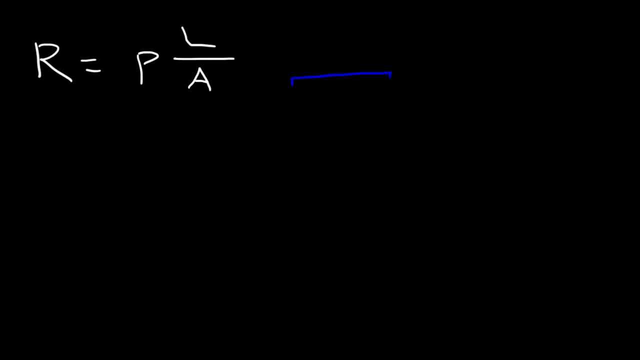 will have more resistance? A short wire or a long wire? What would you say? It turns out that the long wire has more resistance. Now, why is that the case? Well, as you increase the length of a wire, the resistance will increase. if you look at 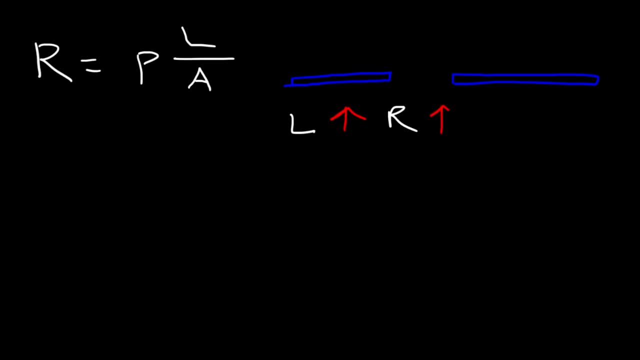 the formula. Notice that L is on the top of the numerator. Whenever you increase the numerator of a fraction, the entire value of the fraction increases. So as you increase the length of a wire, the resistance of that wire will increase. Now here's another question for you: Which wire has more resistance, A thin wire or a? 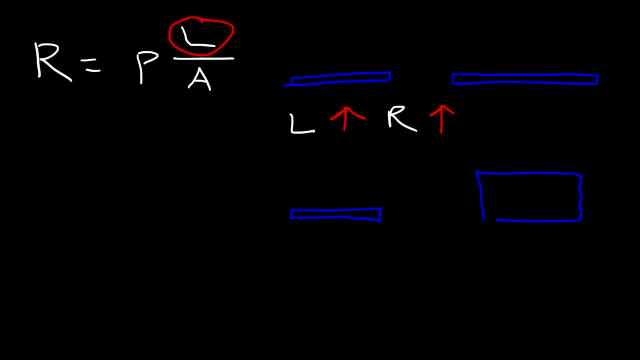 thick wire. And let's say they are. they have the same length. Which one has more resistance? It turns out that the thin wire has more resistance than the thick wire. Looking at the equation, the area is on the bottom. As you increase the cross-sectional area of a wire, the resistance will decrease Whenever. 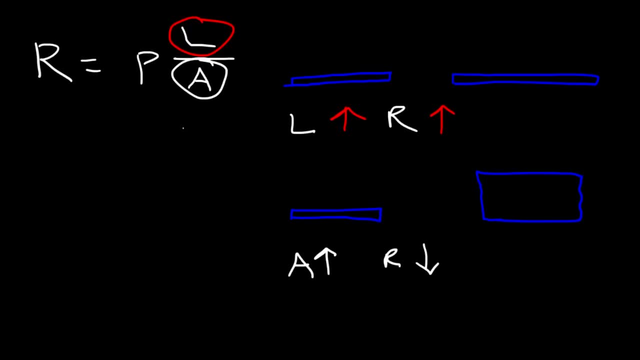 you increase the value of the denominator, the value of the whole fraction decreases. Now, if you think about it, the reason why the thick wire has less resistance is because there's more space for the electrons to move, And because there's more resistance in the space, that conductor can carry more electrons, And so more. 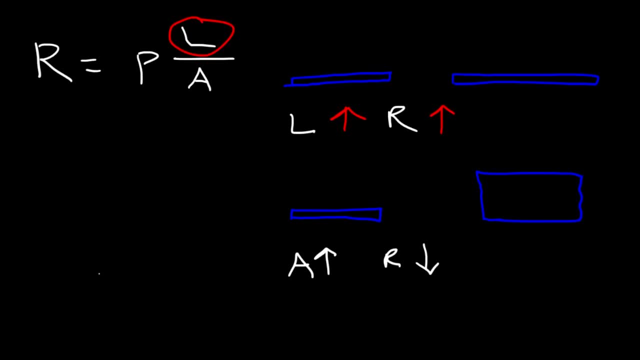 electrons can flow. If there's more current, there's less resistance given the same voltage. Now you can think of it as a highway, The thin wire. think of it as a one-lane highway. There's not many cars that can pass through a one-lane highway. 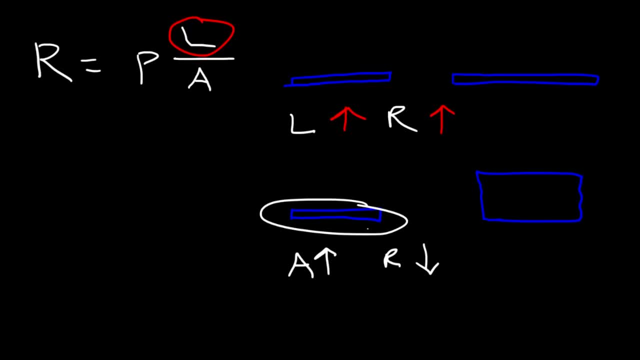 So there's a lot more resistance in a thin wire. But in the thick wire imagine it as a seven-lane highway. More cars can flow through a seven-lane highway And so there's less resistance. In the case of length, the longer the road, the more time it's going to take to get through it. So if you increase, 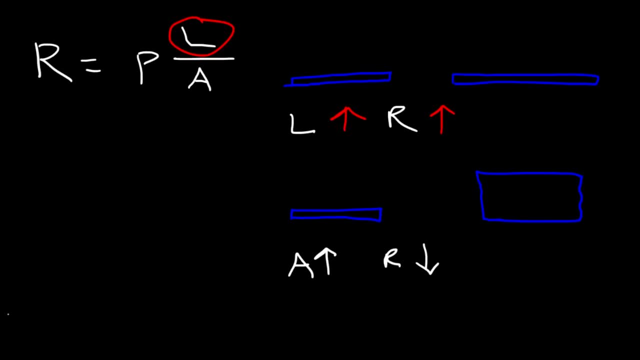 the length, the resistance will increase. Now, what about P, the resistivity? What does that tell us? That is a property of the metal itself or the material that conducts electricity. In the case of a good conductive wire, the resistance will increase. In the case of a good conductive. 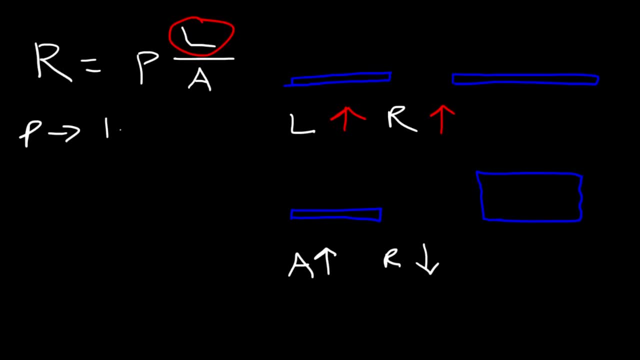 wire like a metal. the resistivity is in the range of 10 to the minus 8.. It's pretty low. Metals have low resistance, which means that they're very good conductors. Two good conductors are silver and copper. Silver has a 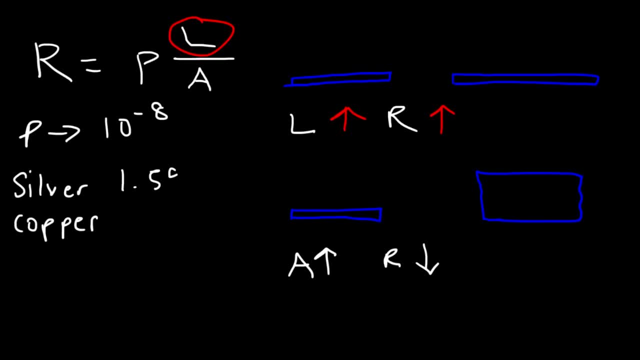 resistivity of 1.59 x 10 to the negative 8, and copper is about 1.68 times 10 to negative 8.. Based on this, which of these two metals is a better conductor, silver or copper? given the resistivity values Now, copper has a higher resistivity than silver. So therefore copper has more resistance. So if copper has more resistance then it's going to conduct electricity a little bit less efficient than silver. So resistivity and conductivity: they're inversely related. Because copper has a higher resistivity it's less conductive, And because silver has a lower resistivity it's more. 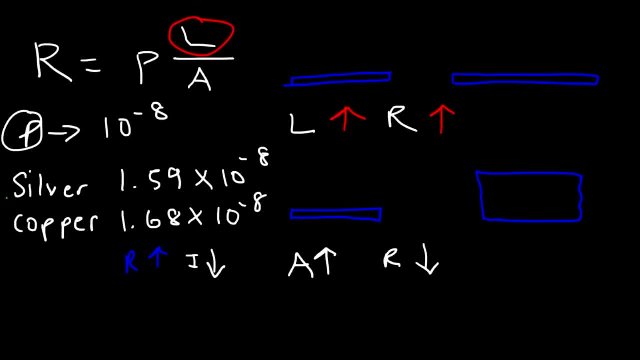 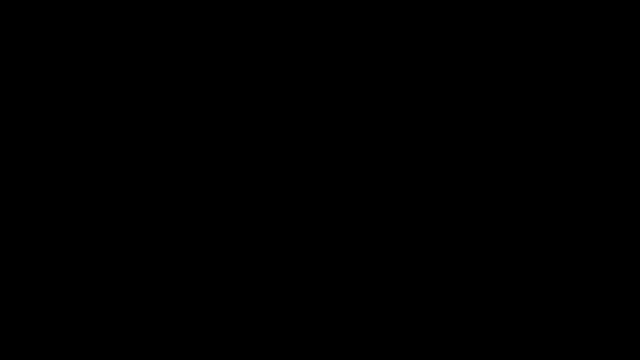 conductive. So silver is a better conductor than copper. So materials with low resistivity means that they're good electrical conductors. Metals typically have a resistivity in this order: 10 to negative 8. Semiconductors or semimetals like carbon, graphite, germanium and silicon, the resistivity is much. 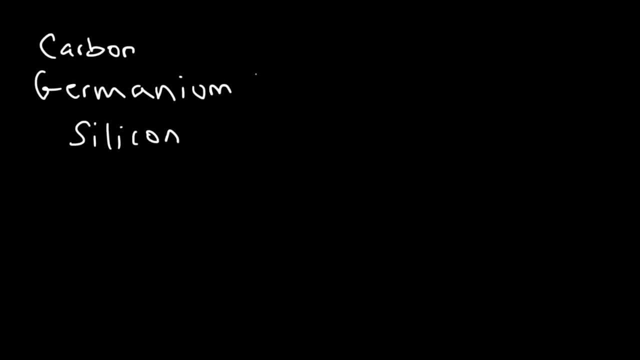 higher. In the case of carbon graphite. it's about anywhere between 3 to 60 times 10 to minus 5. So it's much higher than a typical metal, but it still conducts electricity differently. Fairly decently, it makes good resistors. 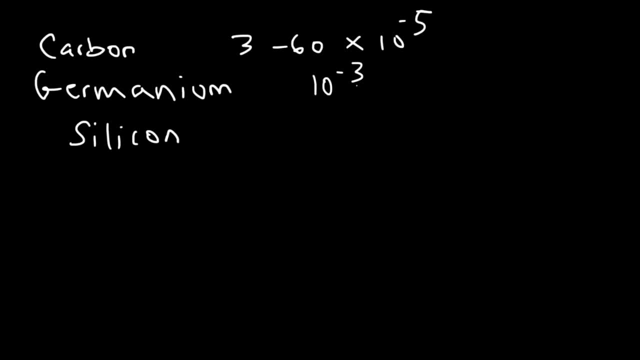 Germanium is on the order of 10 to the minus 3. Silicon anywhere from 10 to the minus 1, to 10 to the 1. So silicon is not a good conductor. for the most part It conducts a small amount of electricity. 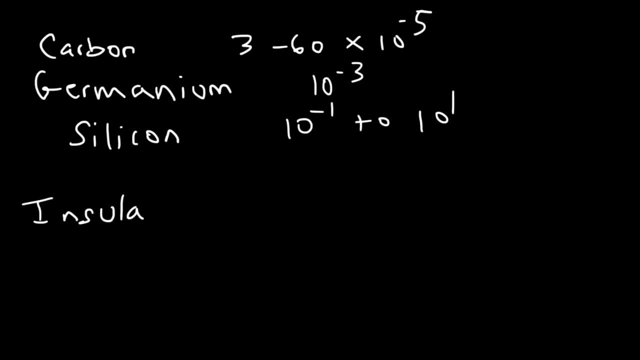 Then you have insulators which for the most part do not conduct electricity. So glass has a resistivity but it conducts less than 3 to the minus 5 times 10 to the minus 3.. that's very high. 10 to the 9 to 10 to the 12. That's a lot higher than silicon. 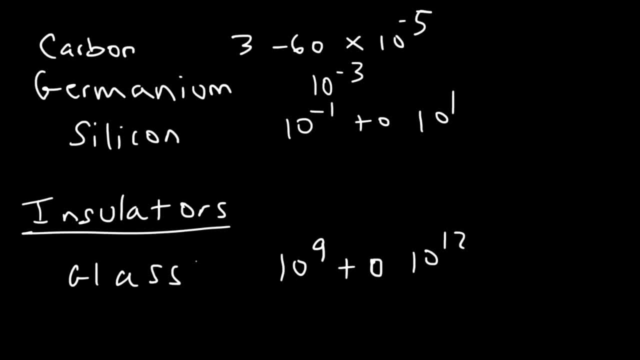 So for the most part, insulators, they just don't conduct electricity. Semiconductors, they conduct a small amount of electricity. And metals: because they have such low resistivity values, they're very good conductors of electricity. Now, resistivity is a function of temperature. 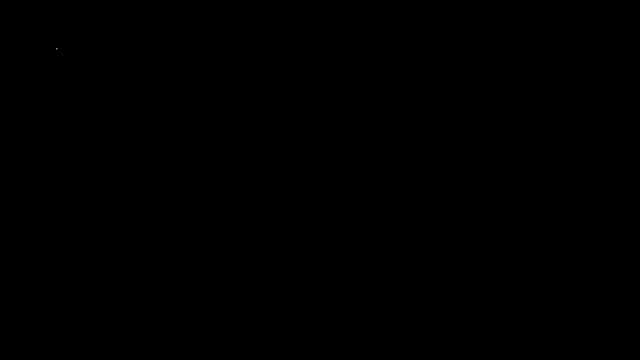 There's an equation that you need to know, and here it is: PT is equal to PO times 1 plus alpha, T minus TO. So this means that the resistivity of a metal is affected by the temperature. Now the situation is different for semiconductors. 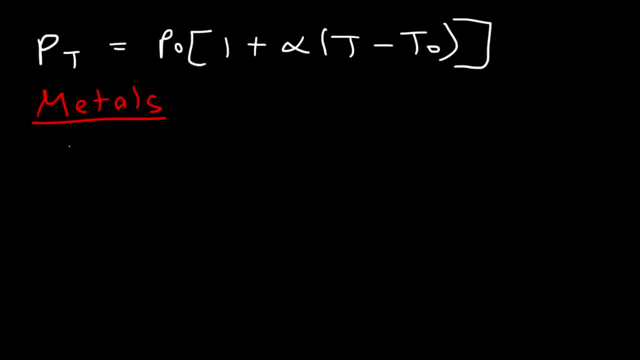 For metals. as you increase the temperature of the metal, the resistivity decreases. I mean it increases. I take that back. No, it decreases, It increases. Now, why is that the case? Well, whenever you raise the temperature of the metal, the free-moving electrons, they're. 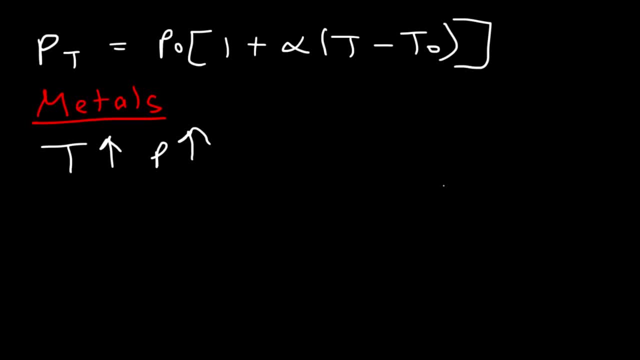 colliding much more frequently, And so the drift velocity of the electrons caused by an electric current is much less. because you have to go against all the random collisions that are occurring inside a metal And, as a result, metals. they have a much higher resistance at higher temperatures than 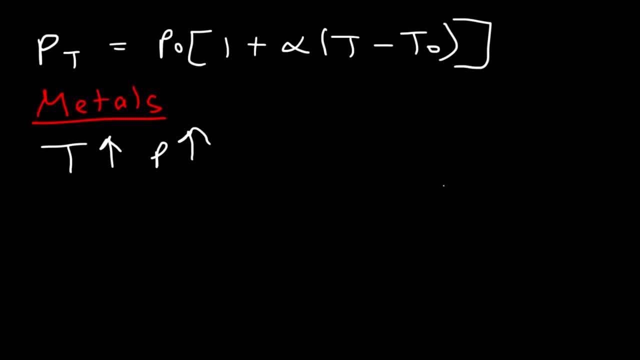 at low temperatures. So metals conduct electricity better at low temperatures rather than at high temperatures. If you cool a metal enough to a very, very cold temperature, a metal can become a superconductor where there's virtually almost no resistance. 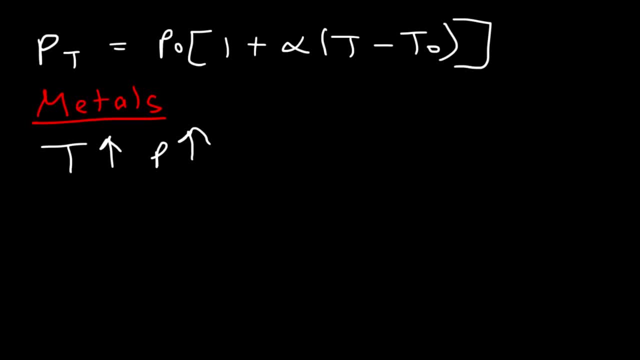 So make sure you understand this. as you increase the temperature, the resistivity goes up, and so they have a higher resistance, which means that they're less conductive at high temperatures. metals conduct electricity better at low temperatures. now, semi-metals or semiconductors like carbon, graphite, silicon, germanium, the 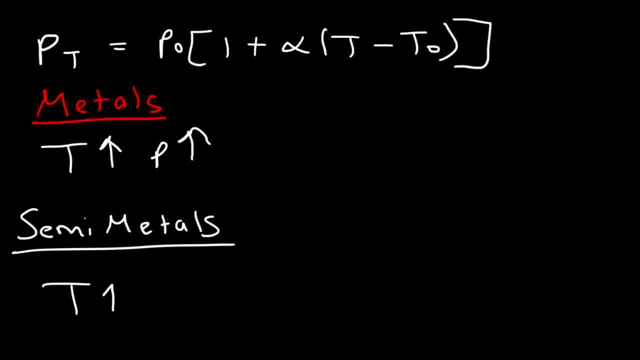 situation is different. as you increase the temperature they become more conductive, they conduct electricity better and the resistivity decreases. so it's different for semiconductors, just keep that in mind. metals: they have a positive temperature coefficient, so alpha is positive, that's the temperature coefficient of resistivity. and because alpha is, 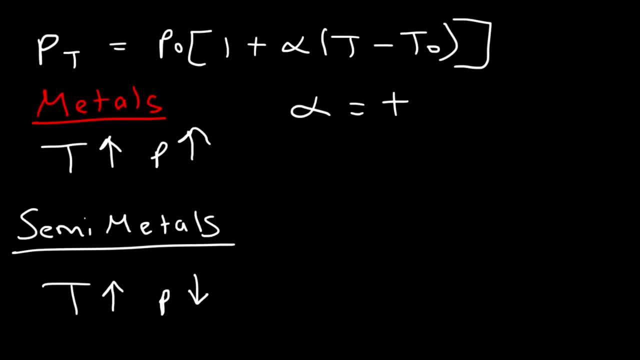 positive for metals. if you can go to your physics textbook and look at the table for resistivity, you'll see that it's positive for metals and you can see that metals they have a positive coefficient of temperature, which means that temperature and resistivity are directly related. if you increase the 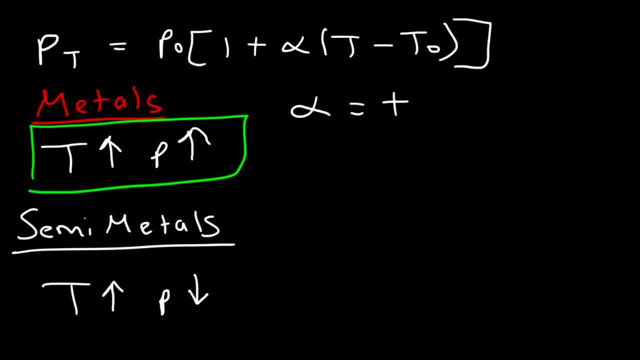 temperature, the resistivity go up for semiconductors. they have a negative temperature coefficient, which indicates an inverse relationship. as you increase the temperature, the resistivity goes down, which means that semiconductors are more conductive at high temperatures, but metals are less conductive at high. 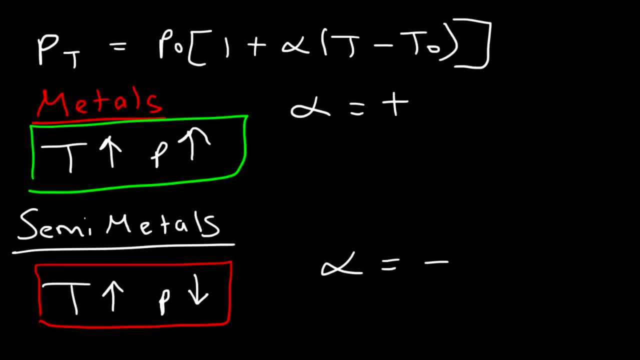 temperatures. so why is this information useful? why do we need to know the relationship between temperature and resistivity? well, sometimes you may want to digitally measure the temperature of an object and you can use a digital thermometer for that, and it's based on this principle: by knowing the resistance. 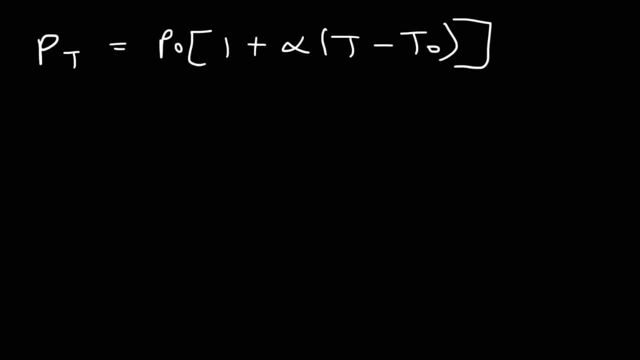 of a metal at a given temperature, and if you can measure the resistance at a new time, you can calculate that temperature based on that new resistance value. out of the ring you get aetric resistenceaquit好. now r is equal to p times L over a. so the ratio between, let's say, our two of our, 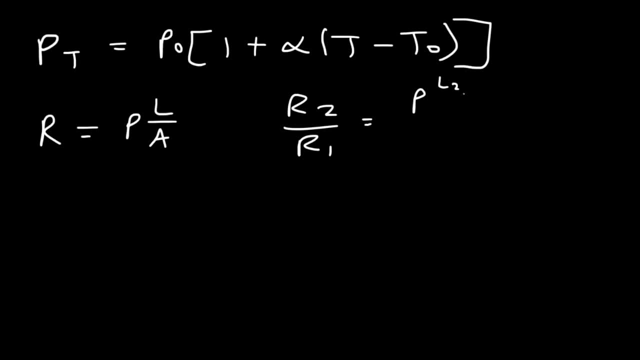 one, that's going to be P, L two over L one. I mean ok. OK. so given your current temperature, our current temperature, we need to equate this pesos. so we're going to calculate R n plus a and that's going to equal to P. choose the value of a times L. over 8 divided by P, 1 times L over a. I didn't put a subscript for position. that is Because when I answered temptation it's not possible. but if I'm Хотя Stewart n is not 1, which I get the result twice times L by 1. so if you try there, toouth even notes 1cı連mos alors. 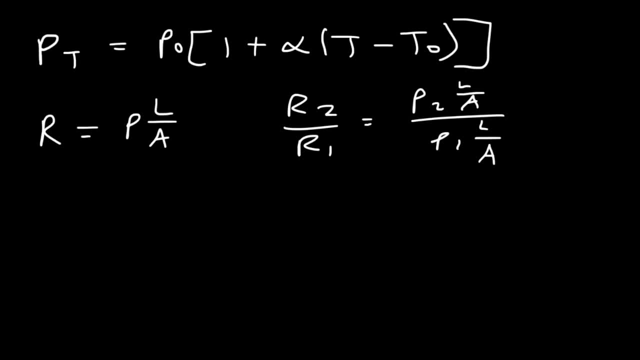 assuming that the wire remains the same, If it has a constant length and a constant area, and if only the temperature changes, then the resistivity will change only. So L and A will be the same, which means that they can be cancelled in this equation. So if we keep the length of the wire and the 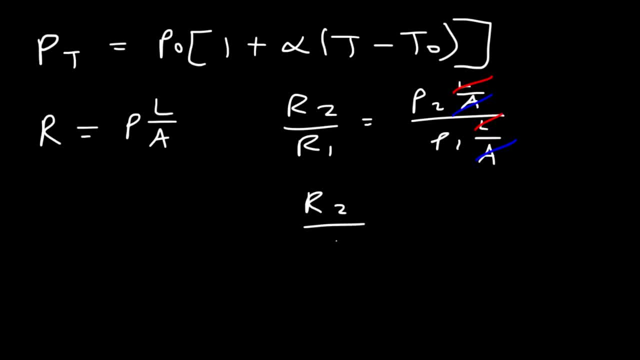 cross-sectional area the same. the resistance will depend on the resistivity And it makes sense: If you increase P, R will increase. So therefore, since this equation is PT over PO or P2 over P1, we can replace it with R2 over R1.. 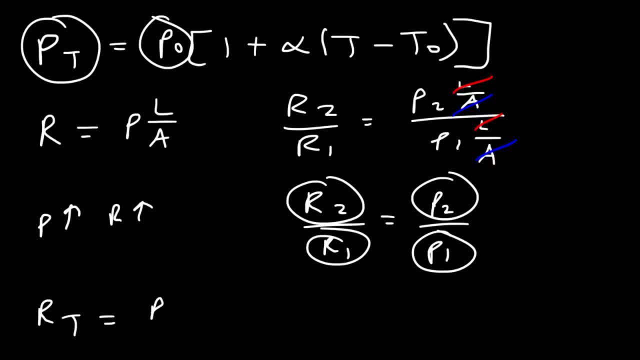 So we can say that RT is equal to RO times 1 plus alpha T minus TO. So if we have the resistance at one temperature, we can say that R2 over R1 is equal to R2 over R1.. So if we have the resistance at one temperature, 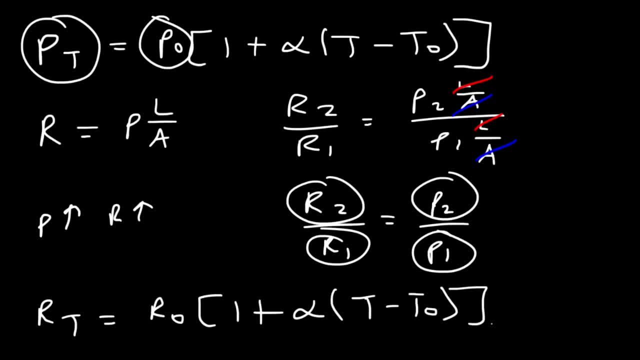 we can say that R2 over R1 is equal to R2 over R1.. So if we have the resistance at one temperature and if we can measure the resistance at a new temperature, then using this equation, we can calculate the new temperature or we can calculate the new. 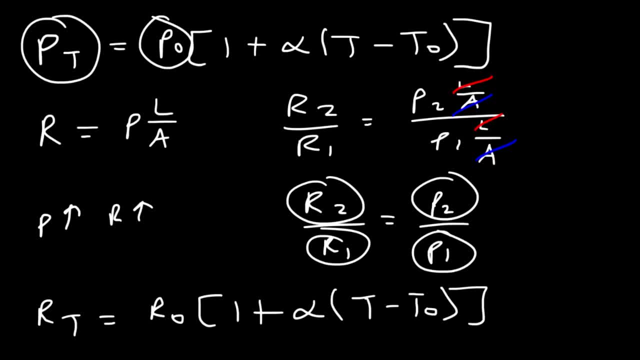 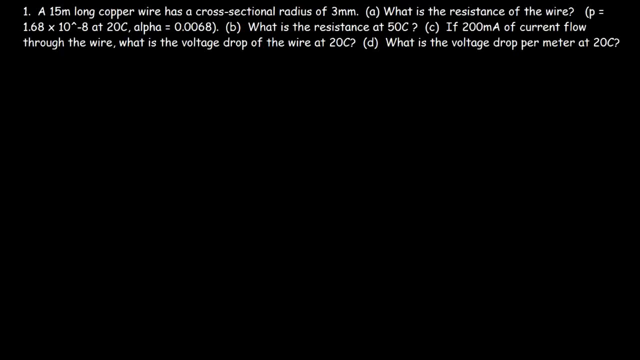 resistance, whichever we want, And so that's how you can use resistance to measure the temperature of an object, or even the temperature of a room, using a digital thermometer. Now let's work on some problems. A 15 meter long copper wire has a cross-sectional radius of 3 millimeters. What is the resistance of the? 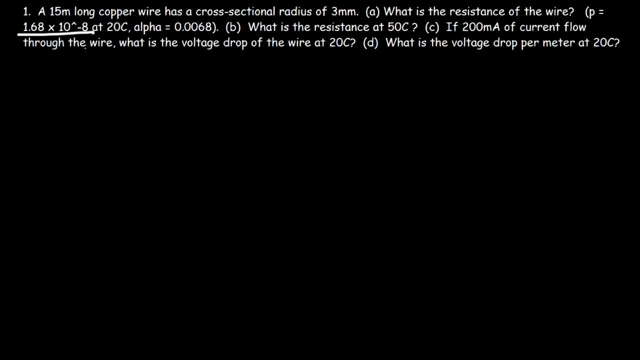 wire And we're given the resistivity, which is 1.68 times 10, to the minus 8 at 20 degrees Celsius, And we also have the temperature coefficient, which is 0.0068.. The equation that we need is this one: R is equal to P times L divided by A. Now let's draw a picture. 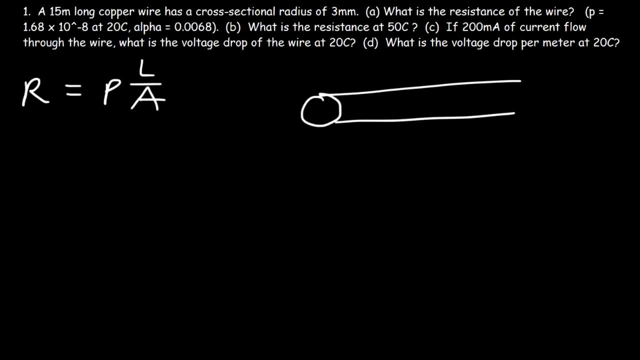 So let's say this is the wire and L represents the length of the wire And this is the length of the wire And here is the radius of the cross-sectional circle that we see here And the area of that is pi R squared. So plug in everything into the 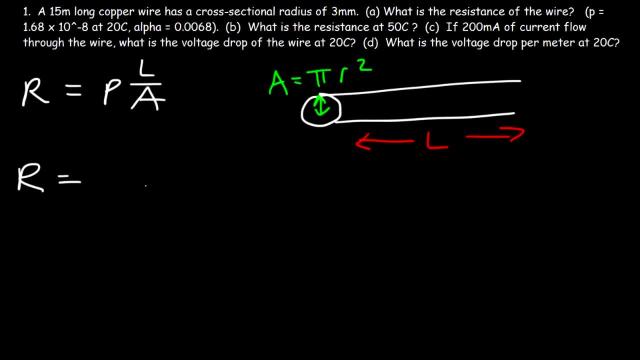 formula Big R, which is a resistance, is equal to the resistivity, and that's 1.68 times 10 to the minus 8, multiplied by the length of the wire, which is 15 meters, divided by the cross-sectional area, which is pi times the radius squared. Now, the radius is 3. 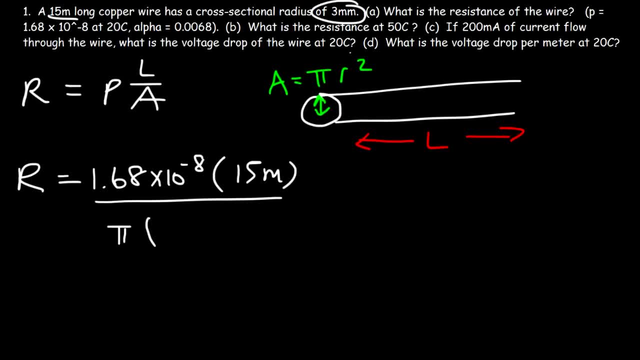 millimeters and you need to convert that to meters. To convert millimeters to meters, you can divide by a thousand, you can move the decimal point three units to the left, or you can simply write 3 times 10 to the minus 3.. Just add 10 to. 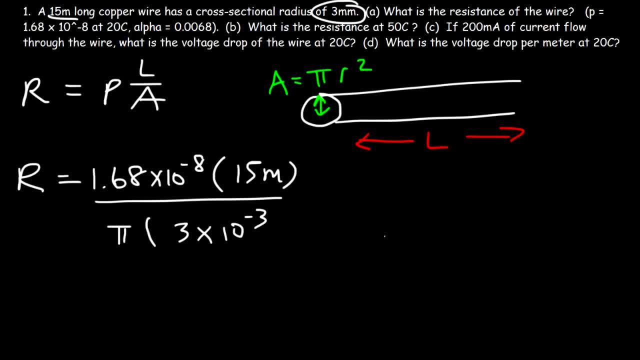 negative 3 for millimeters, because milli represents 10 to the minus 3.. And don't forget to square it, So you should get 0.008913 ohms. If you're having issues getting this answer, make sure you put this in parentheses, Otherwise. 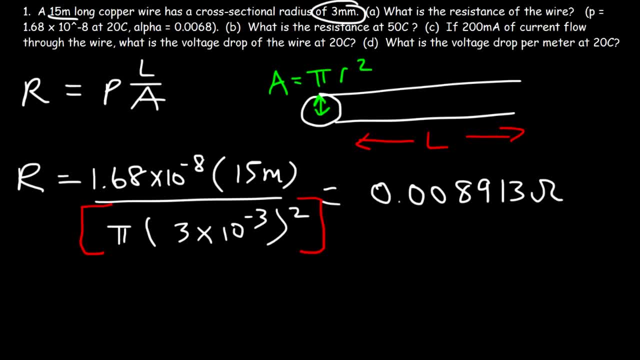 you're going to have a problem. Calculator might divide by pi and then multiply by 3 times 10 to the minus 3 squared Part B. What is the resistance at 50 degrees Celsius? Now what equation can we use to find a new resistance at a higher temperature? We can use this: 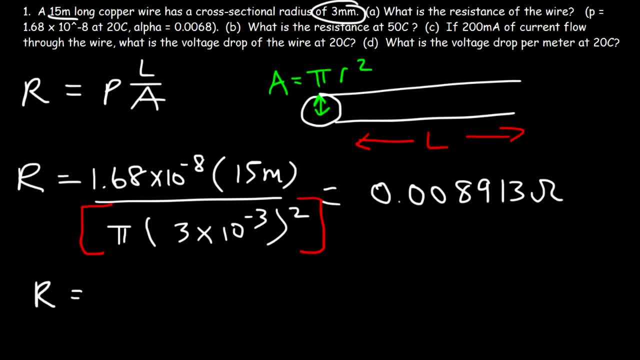 equation R is equal to the original R value multiplied by 1 plus alpha times T minus 3.. T naught or the original temperature. So the resistance at 20 is 0.008913.. Alpha, the temperature coefficient of resistivity, that's 0.0068.. That was given. 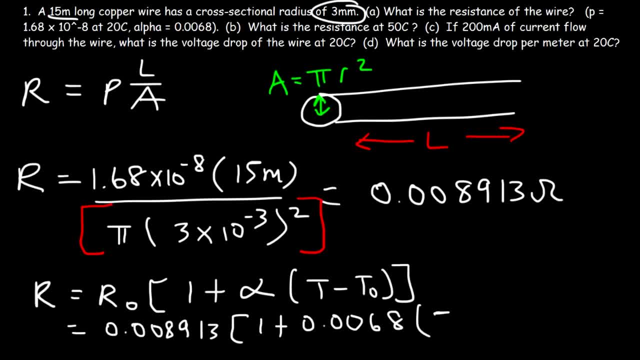 to us in the problem T is a new temperature, that's 50.. To the original temperature which corresponds to this resistance is 20.. So what you want to do in order to get the answer first, subtract 50 and 20, which is 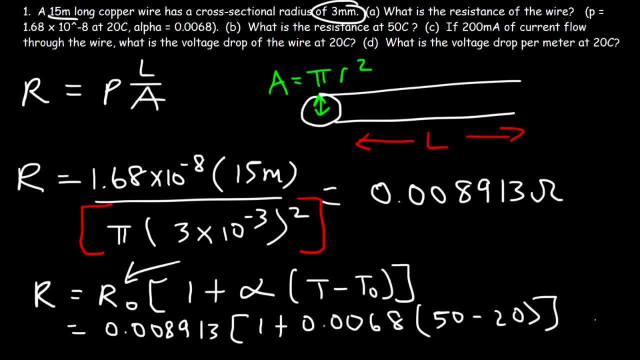 30, and then multiply 30 by 0.0068.. You should get 0.204.. Add 1 to it and then multiply that by 0.008913.. And this is equal to 0.01073.. Now does this answer make sense? 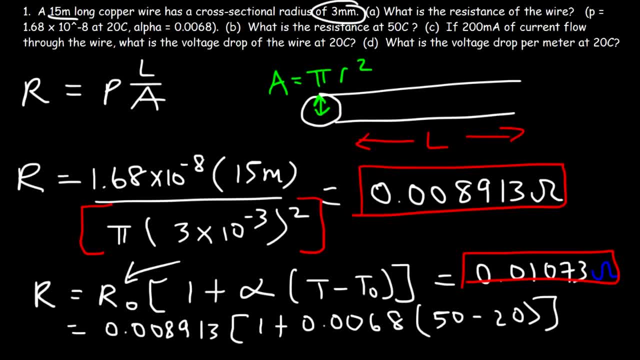 Well, the temperature was increased from 20 to 50.. Any time the temperature goes up, the resistivity of a metal will go up, so the resistance will increase, And that's what we see here. 0.01 is higher than 0.0089.. So as the temperature went up, the resistance. 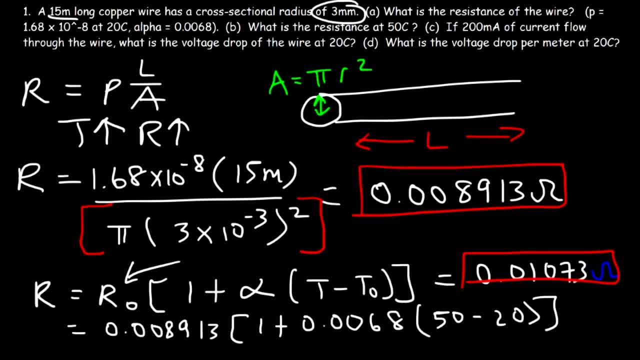 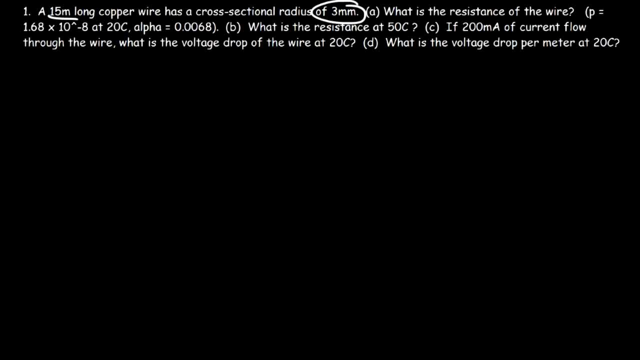 of the copper metal went up as well. Now let's move on to Part C. If 200 milliamps of current flow through the wire, what is the voltage drop of the wire at 20 degrees Celsius? The voltage drop is equal to the product of the current times, the resistance, The current. 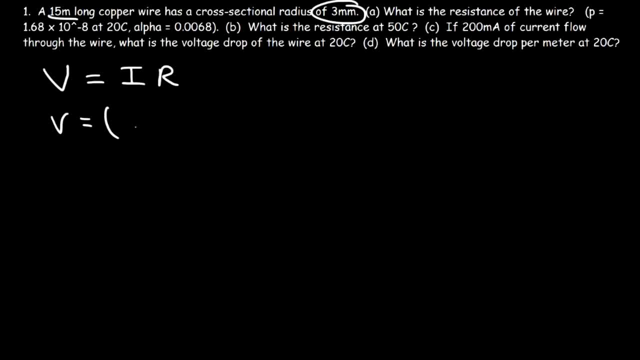 is 200 milliamps, but we need to convert that to amps, So you've got to divide it by 1000.. So that's going to be 0.02 amps and a resistance at 20 is 0.0089.. 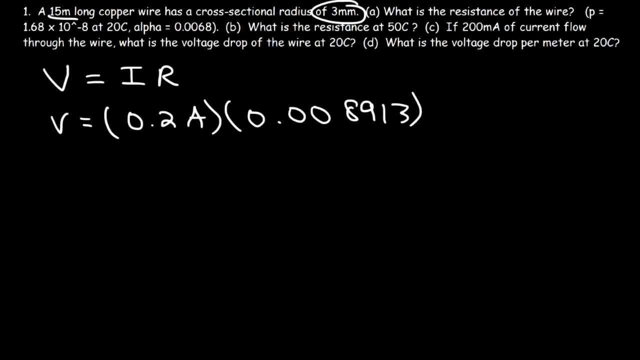 So the voltage drop is .0017826 volts. So this is the voltage drop per 15 meters. because that's the length of the wire And because the number is so small, let's convert it to millivolts. Let's multiply by 1,000.. 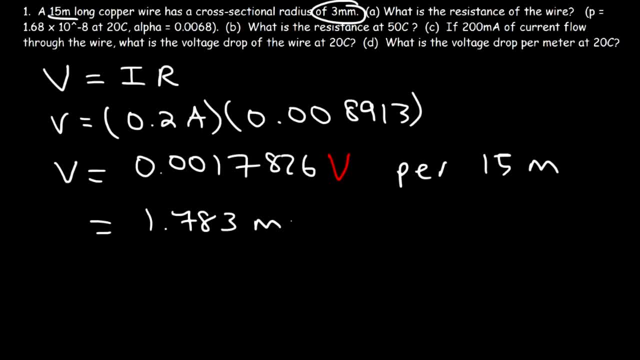 So this is about 1.783 millivolts. Now what about part D? What is the voltage drop per meter? So we need to divide this by 15. And you should get .119 millivolts per meter. With this information, we can calculate the voltage drop at any length. 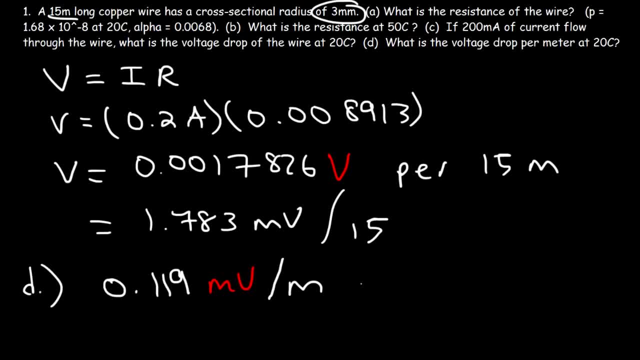 So let's say, if the copper wire was 300 meters long, All we need to do at this point is multiply it by 300 meters, And so these units will cancel, and it's going to be .119,. now this is a rounded answer. 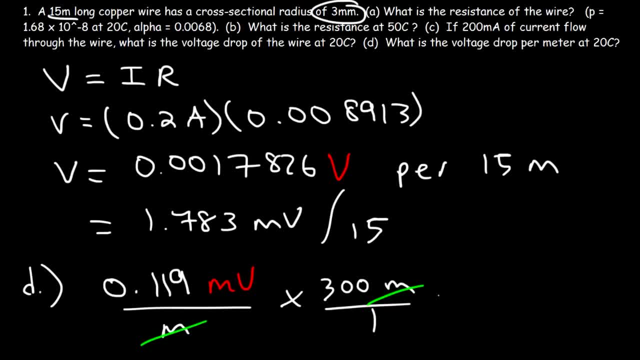 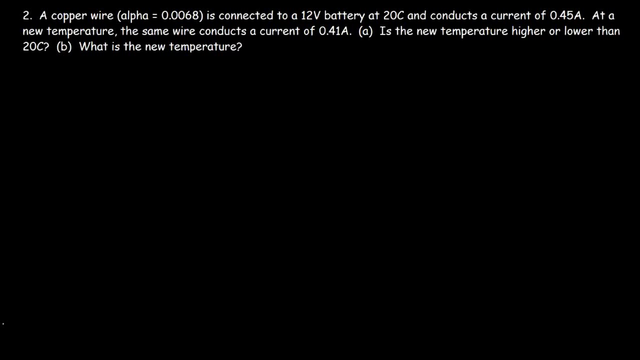 times 300. So the voltage drop is going to be 35.7 millivolts, given a length of 300 meters. So that's it for this problem. Number 2.. A copper wire is connected to a 12-volt battery at 20 degrees Celsius and conducts a current. of .45 amps At a new temperature. the same wire conducts a current of .41 amps. Is a new temperature? Is a new temperature? Is a new temperature higher or lower than 20?? Well, the current decreased as the temperature changed. 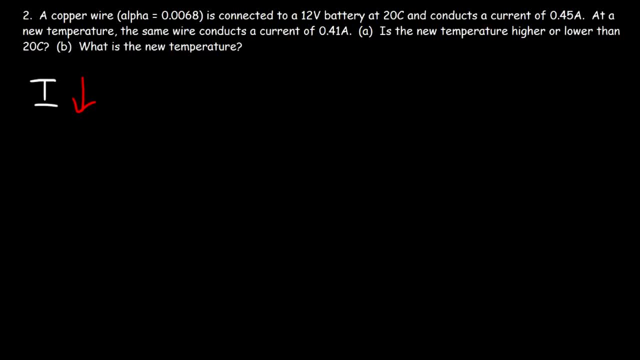 Which means the copper wire is less conductive and so its resistance is greater. The resistance of metals will only increase if the temperature increases, So therefore the new temperature is higher than 20 degrees Celsius. Now let's go ahead and calculate it. So first we need to calculate the resistance at these two different temperatures. 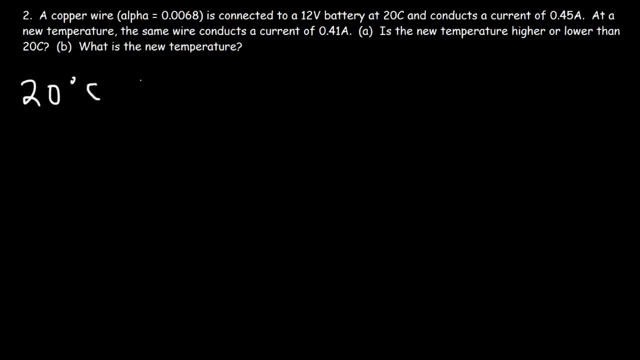 So at 20 degrees Celsius we can use the equation: V is equal to IR, Where R is basically V divided by I, So the voltage is 12 volts and the current at 20 degrees Celsius is .45 amps .45.. .45.. 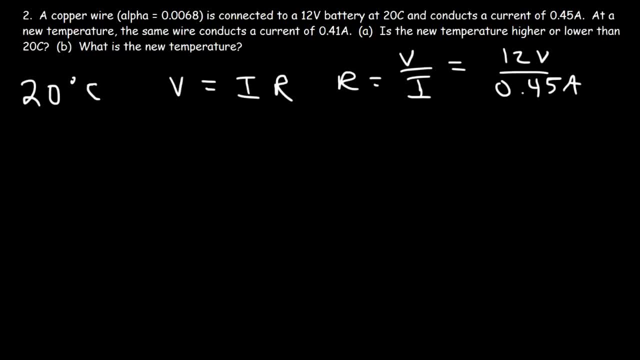 .45.. so 12 divided by 0.45 will give us an R value of 26.667 ohms. now let's calculate the R value at a new temperature. so the voltage is still 12, but the new current is 0.41. 12 divided by 0.41 is 29.268. so that's the 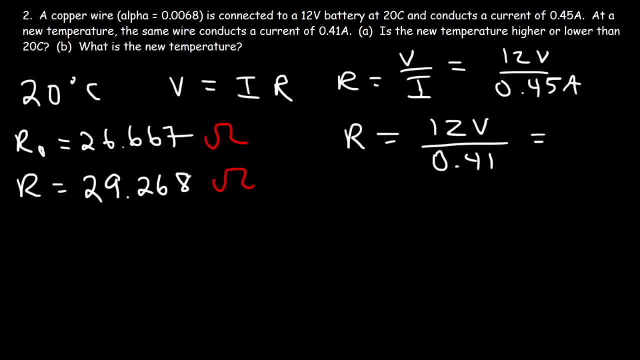 resistance at the new temperature. the equation that we can use to find the new temperature is this equation. so the new R value is 29.267 ohms R O. the original R value is 26.667. alpha is 0.0068 for the copper wire we're. 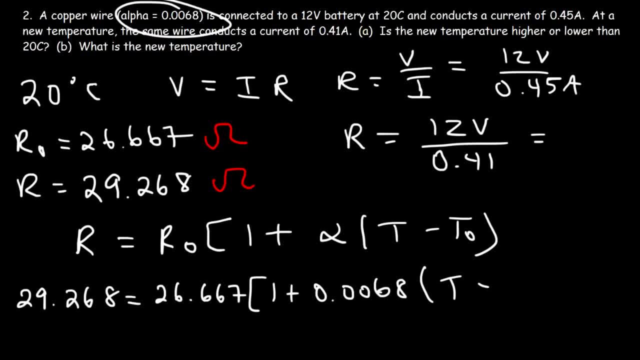 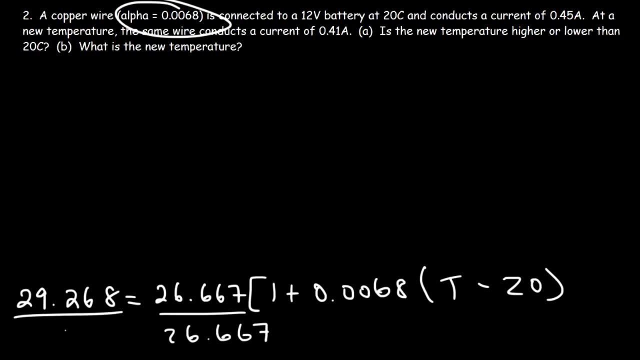 looking for the new temperature T. the original temperature that corresponds to this resistance is 20, so now we just need to do math and solve for T. so the first thing we should do is divide both sides by 26.667. if we do that, we can get rid of the brackets that we have here. so 29.268 divided by 26.667. 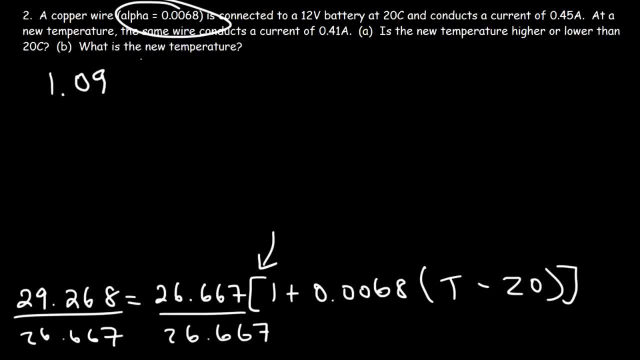 that's 1.09 754 and that's equal to this. next, let's subtract both sides by 1, so point 0, 9, 7, 5, 4 is equal to point 0 0, 6, 8 times T minus 20. after that let's divide both. 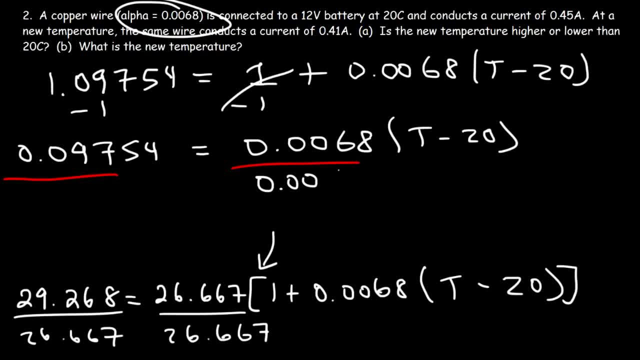 sides by point 0, 0, 6, 8, 0.09 754. divided by 0.00 6, 8, that's equal to 14. point 3: 4 and that's equal to T minus 20. so the last thing that we need to do is add 20 to both sides to. 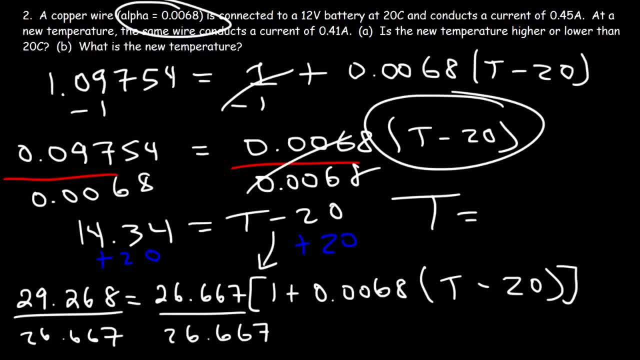 isolate T, so the new temperature is 20 plus fourteen point three four, so it's thirty four point three four, And that is the final answer. That's how you can calculate commute temperature given two different currents.